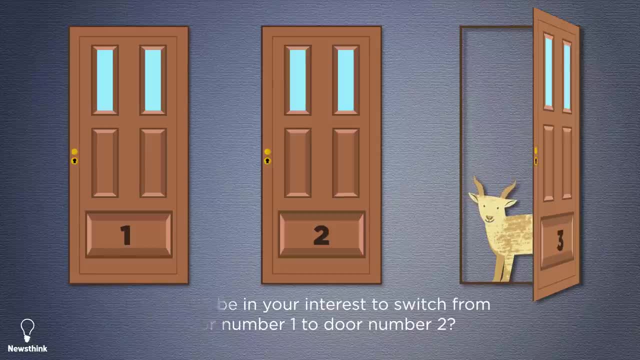 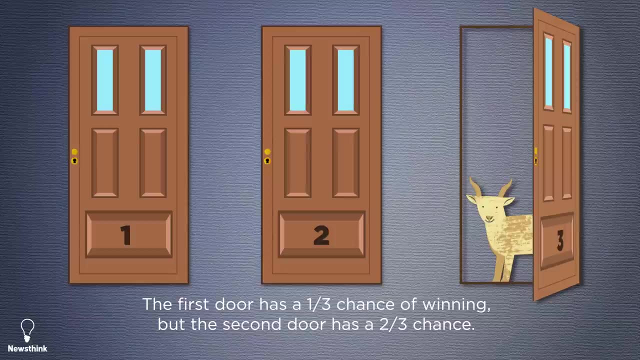 so they don't see the benefit of switching. However, Vos Savant replied: yes, you should switch. The first door has a one in three chance of winning, but the second door has a two in three chance. She got so much heat for this response and couldn't have imagined the backlash that would follow. 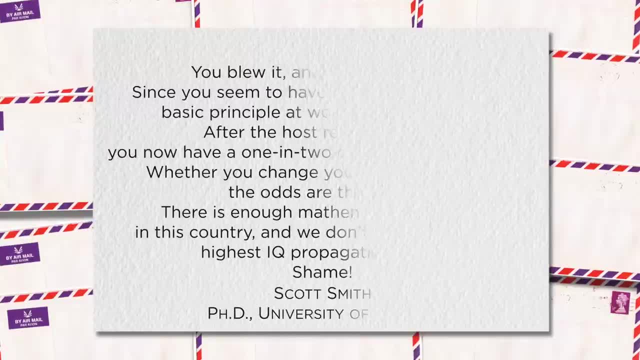 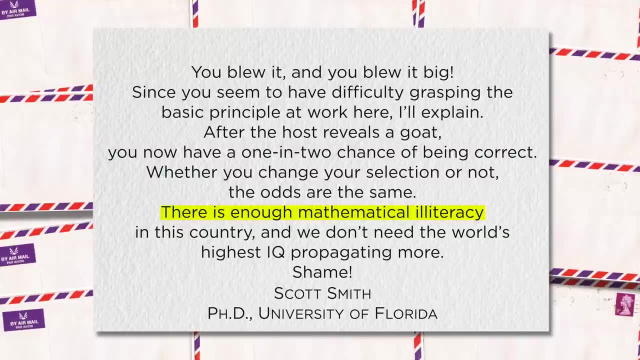 She received thousands of angry letters and said 90% of them told her she was wrong. Scott Smith, who has a PhD from the University of Florida, wrote: There is enough mathematical illiteracy in this country and we don't need the world's 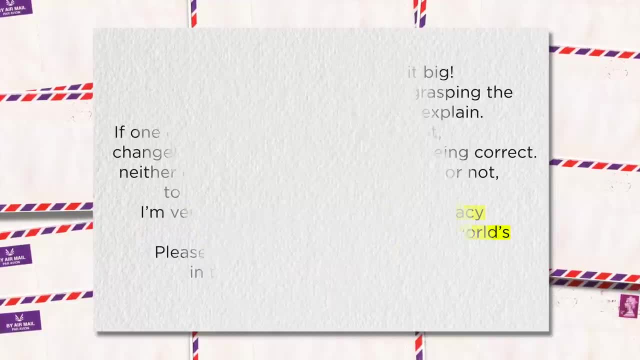 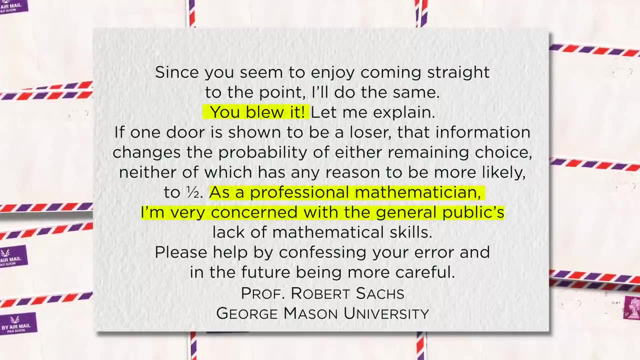 highest IQ, propagating more Shame. Here's a letter from Professor Robert Sachs of George Mason University. You blew it. As a professional mathematician, I'm very concerned with the general public's lack of mathematical skills. Please help by confessing your error and, in the future, being 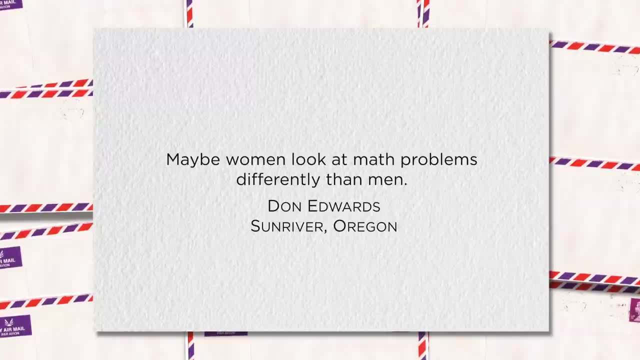 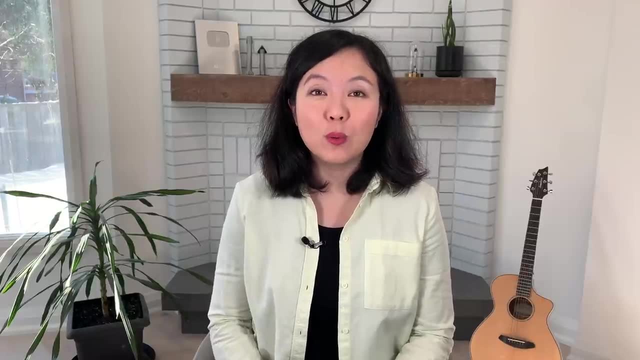 more careful. Don Edwards of Oregon put it this way: Maybe women look at math problems differently than men. But actually the people who sent her the not-so-friendly letters were absolutely wrong. Switching your door does increase your probability of winning the prize When you first choose door. 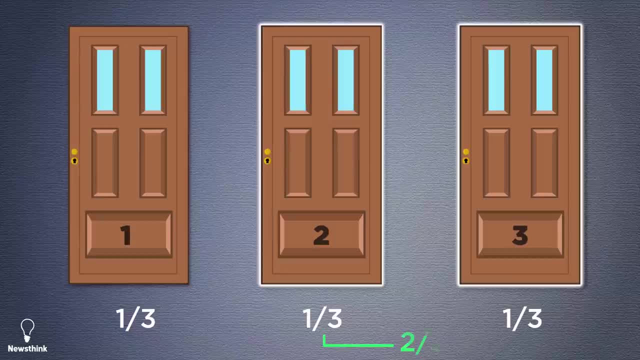 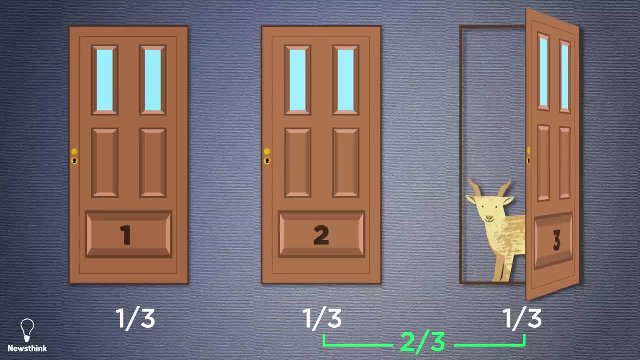 number one. there's a one in three chance that the prize is behind that one and a two in three chance that it's behind one of the other two. But then the host steps in and gives you some help by opening up the door they know is a loser. So door number two must have the rest of the prize. 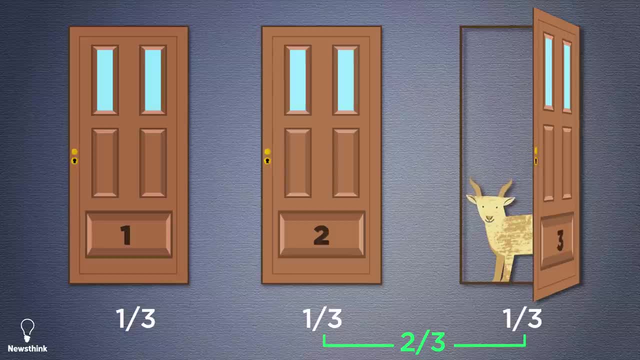 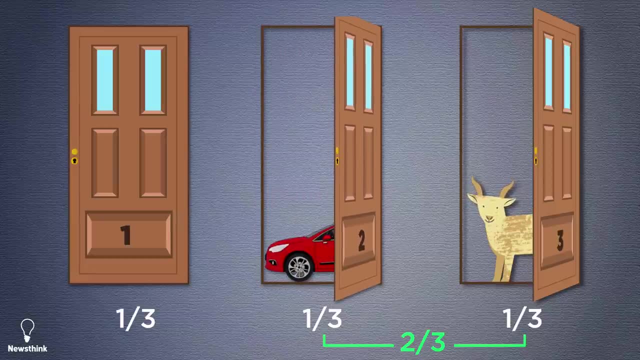 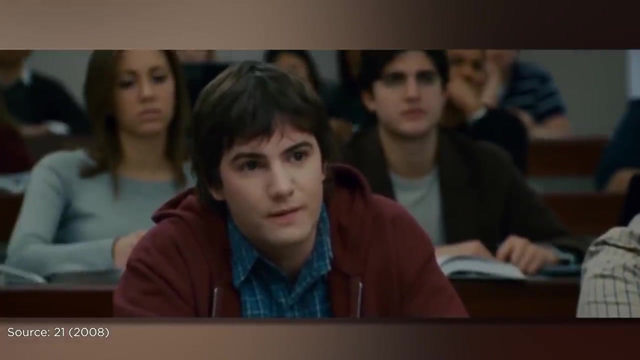 It went from having a one in three chance to a two in three shot at the prize, since the host filtered out the bad door for you. door number three: Switching doubles your odds of winning, Or put another way. So yeah, I'll take door number two and thank you for that extra 33.3%. The outcry: 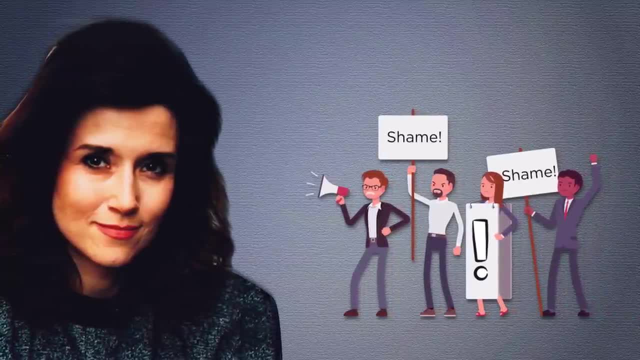 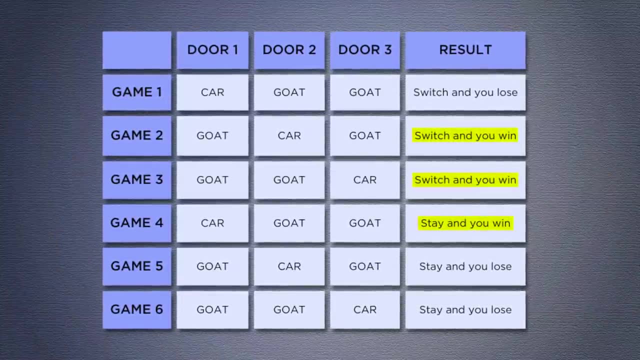 against Vassevan was so extreme that she felt compelled to devote several other columns to explaining her logic. She noted that the benefits of switching can be proven if you were to play through the six games that exhaust all possibilities. This is contingent on the host always opening a door with a goat Mapping out all the possibilities. 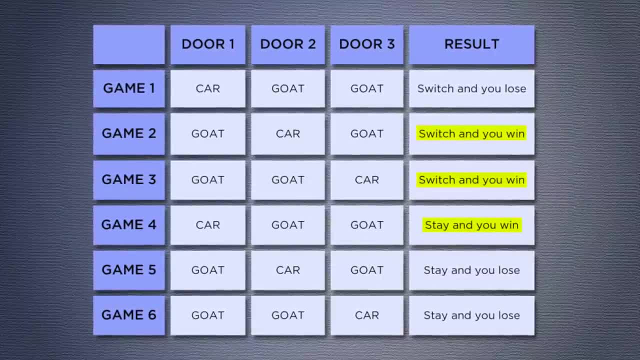 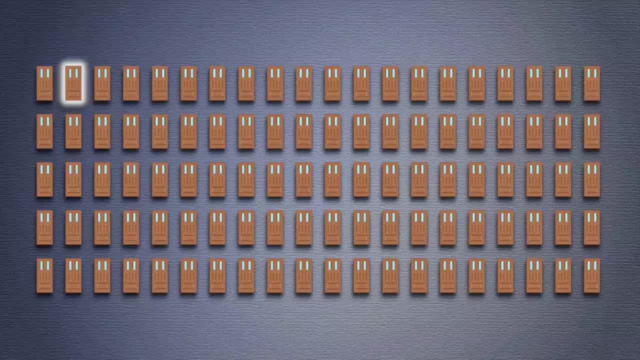 shows there's a higher chance of winning if you switch than if you stay. It's easier to understand the problem if there are many more doors. Say, you chose one door out of a hundred. The host then eliminates 98 doors that they know don't have a prize behind them. That leaves two doors: the one. 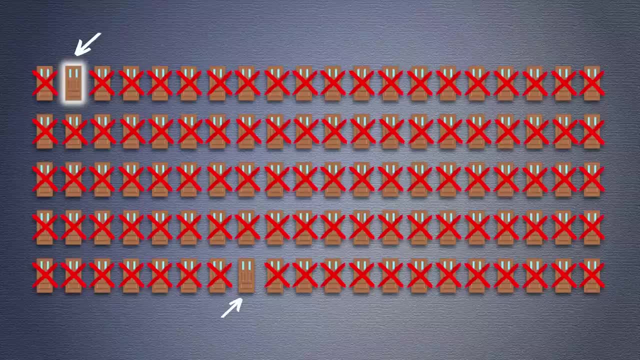 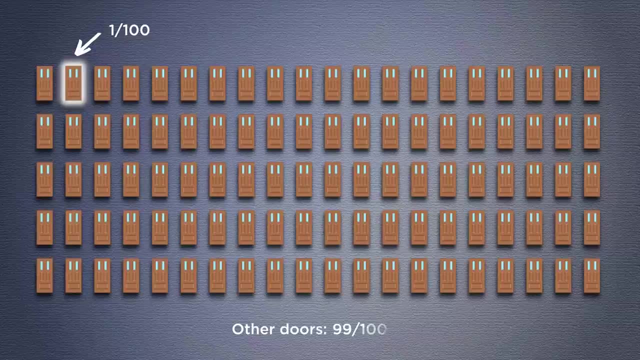 you chose and the only other one remaining. Do you switch now Absolutely? When you first picked, you only had a one in one hundred chance of getting the right door. The odds of it being behind the other doors was 99 out of a hundred. The host then filters out the options. 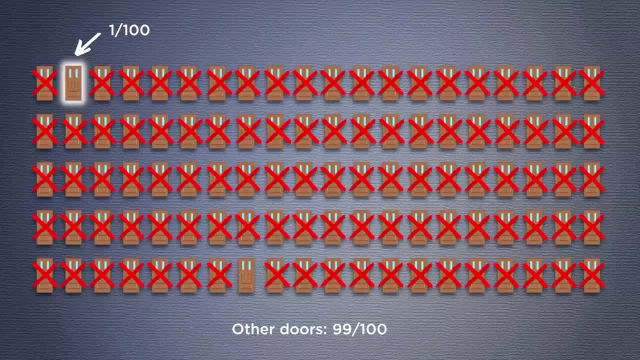 for you by eliminating 98 bad doors that they know don't have the prize. This is to your advantage because it leaves the remaining door with the rest of the odds: A 99 out of a hundred chance of having the car. Some eventually admitted they were in the wrong. A team at the Massachusetts 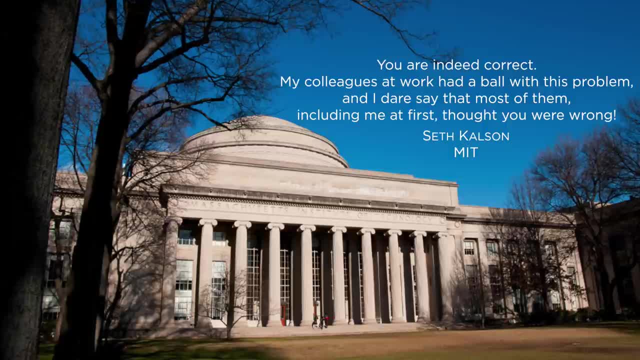 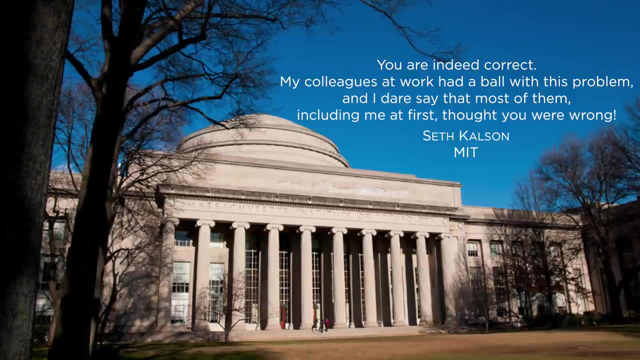 Institute of Technology worked on the problem and afterwards Seth Coulson of MIT admitted: you are indeed correct. My colleagues at work had a ball with this problem And I dare say that most of them, including me, at first, thought you were wrong, To which she. 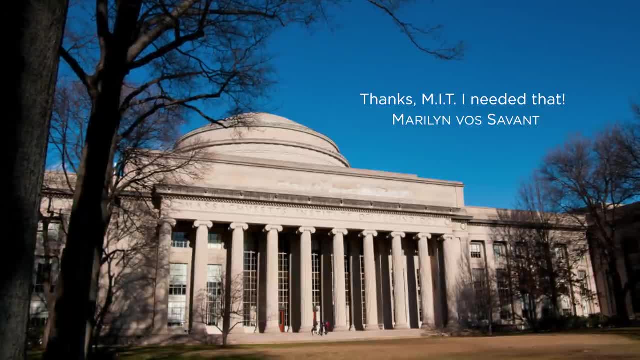 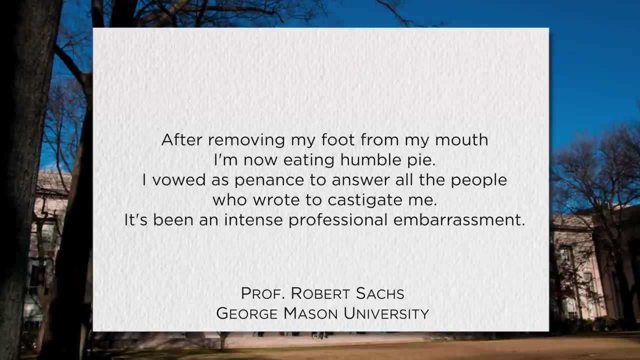 responded. thanks, MIT, I needed that. As for that math professor I mentioned earlier who sent that not so friendly letter, Professor Sacks later conceded, after removing my foot from my mouth, I'm now eating humble pie. I vowed as penance to answer all the people who wrote to castigate me. 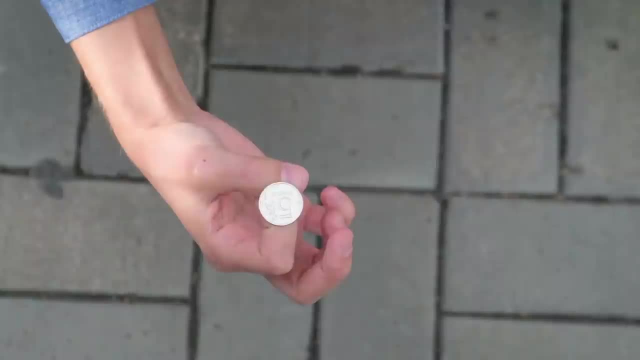 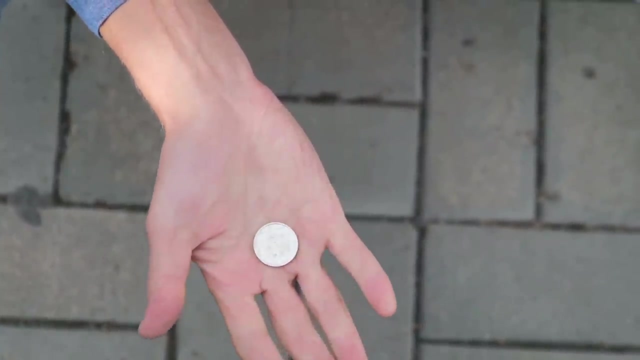 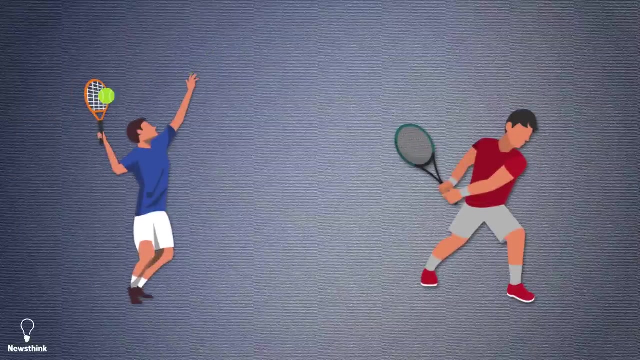 It's been an intense professional embarrassment. Our biggest misconception is assuming that two choices mean a 50-50 chance of something happening. This makes sense if we don't have any other information. If I picked two people and asked who would win a tennis match and you don't know anything about them, you have a 50-50 shot of. 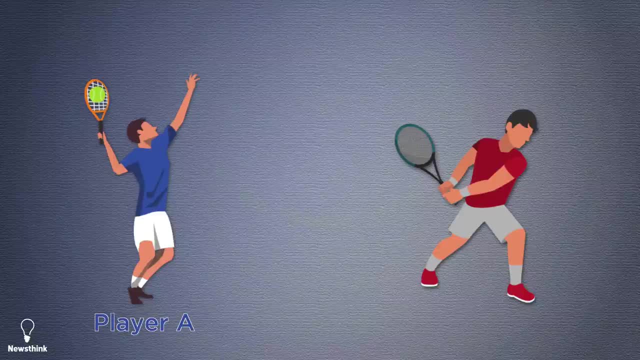 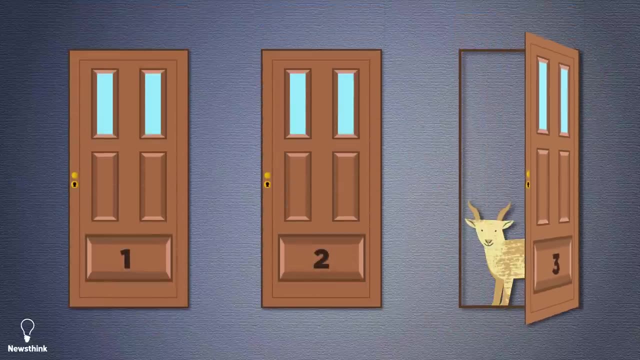 getting it right. But if I said player A just took up the sport yesterday and player B has won Wimbledon, this would likely change your choice. Information matters, Just like when the game show host knew which door had a goat. they weren't opening up a door randomly, So the more you know. 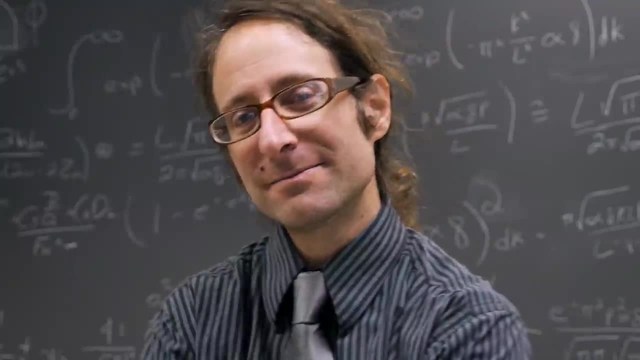 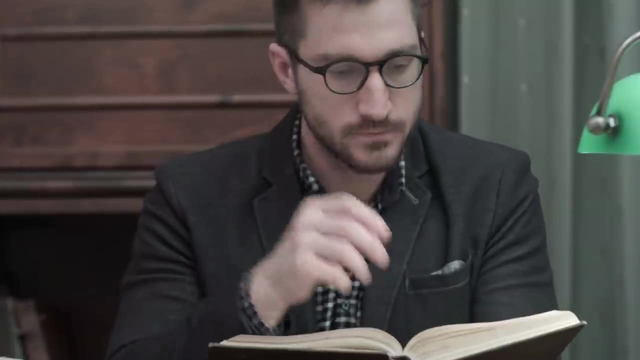 the more informed decisions you can make. Vassevant once said: 教育- Since growing up in the US, there's really been very few things인, She explained. they're more likely to be educated or experienced rather than intelligent. What does she think is holding people back from? 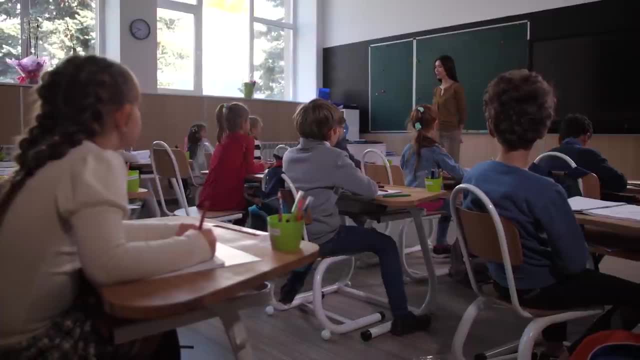 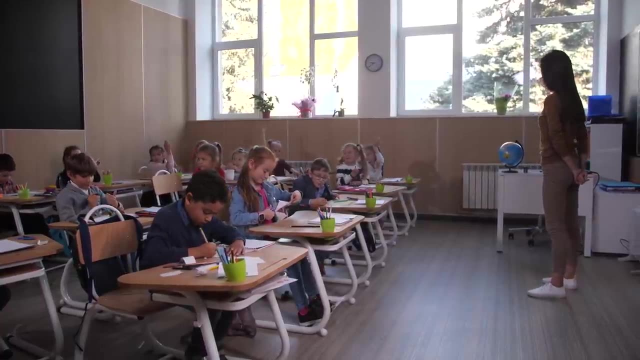 their intellectual potential. Vasseérer and a senior student, she's been critical of compulsory schooling because she says students learn passively. They sit there and are told what to believe instead of learning to think independently. She went so far as to say I would rather not see compulsory schooling.